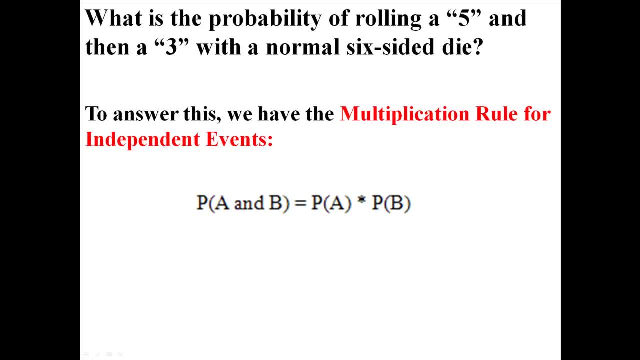 we have the multiplication rule for independent events, Which is the probability of both A and B occurring is the probability of A times the probability of B. So the probability of getting a three and then a five is the probability of three, which is one out of six times the 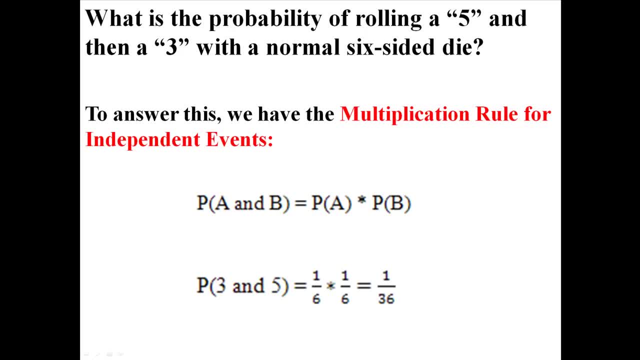 probability of getting a five, which is one out of six. So the probability of getting both a three and then a five is one out of thirty-six, And that is the multiplication multiplication rule for independent events. Now I might want to ask you: what is the probability? 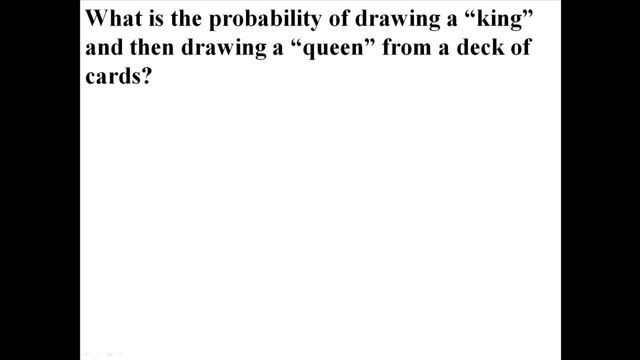 of drawing a king and then drawing a queen from a deck of cards. Now, remember, these are dependent events. So to answer this, we have the general multiplication rule for dependent slash conditional events. Conditional events are basically dependent events And it's something like this: We have the 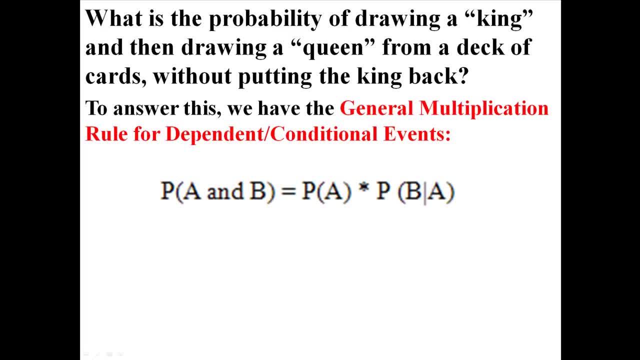 probability of both A and B occurring is the probability of A times the probability of B, given that A has already occurred. That's what that means. So in this case, the probability of getting a king and queen is, first of all, the probability of A is 4 out of 52, because there 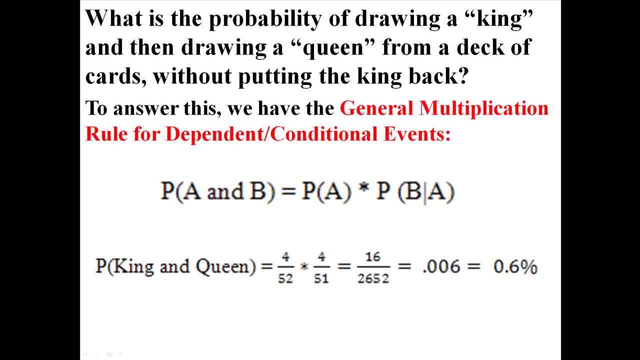 are four kings in the deck of 52 cards, And then the probability of B having drawn A already is 4 out of 51, because there are four queens in the deck, but now there are only 51. Because you've already taken out the king. So you multiply those two things and you get 16. 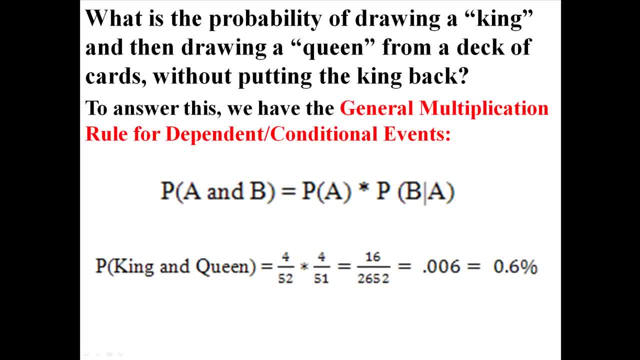 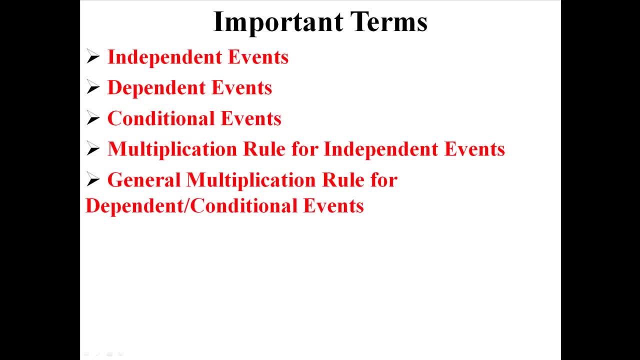 divided by 2,652, which ends up being about 0.6%, There's a 0.6% chance that you will draw a king and then a queen. So that's the multiplication rule for independent and dependent events. So know the difference between independent and dependent events, dependent events and conditional. 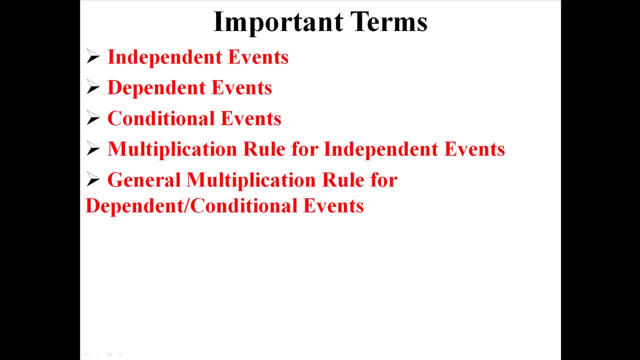 events being basically the same thing, And also understand how to use the multiplication rule for independent events and how to use the multiplication rule for dependent events.